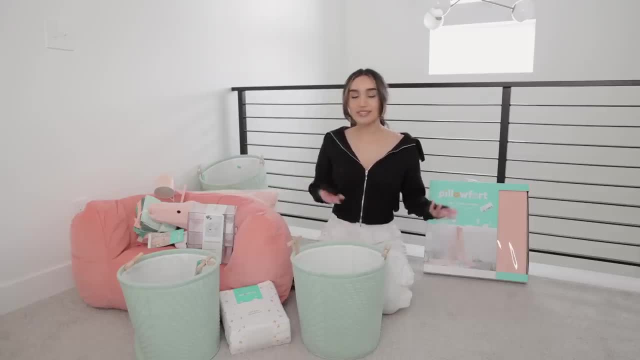 messy too, so I definitely have to organize all of that. so, yeah, I'm really excited to see how their space looks after all these little touches and, of course, the organizing. so, yeah, hopefully this helps you guys out if you guys need to refresh your kids space too. 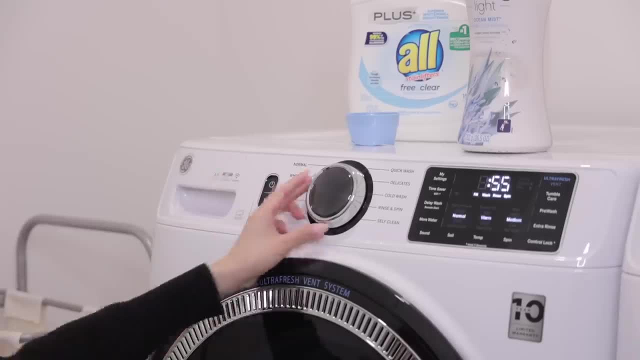 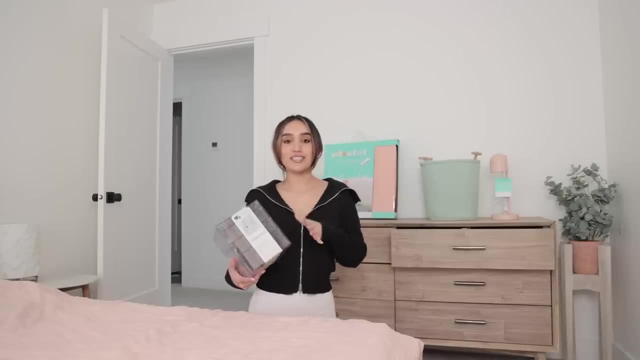 so one thing I did want to organize first is Emma's accessory drawer. this thing is huge but she's sharing with Ember right now and it's just like a disaster. every time I'm trying to get her ready in the morning it's so hard because everything's just like scattered between both. 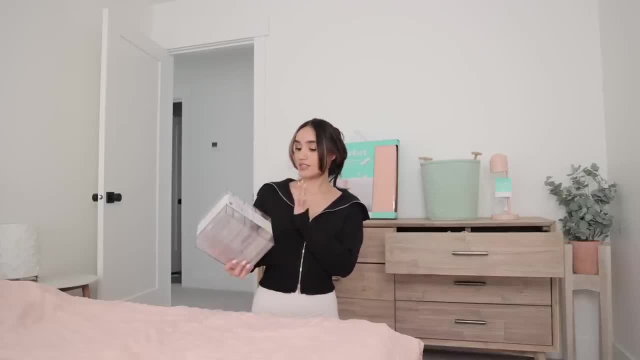 of their stuff. so when I was at Target today I found this four drawer organizer. it's by Bright Room and I really like how small the little one is and I'm going to show you guys how small it is so I can hold, like her brushes down here, maybe some rubber bands and clips, of course, and like a 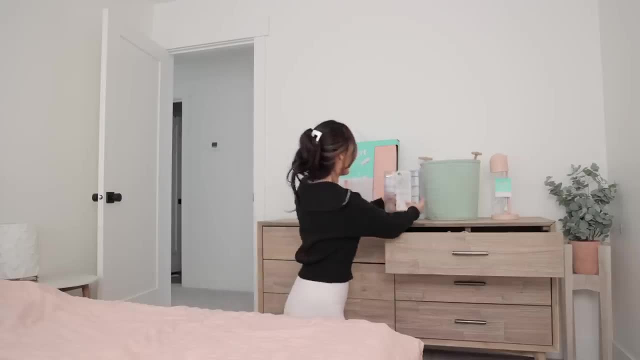 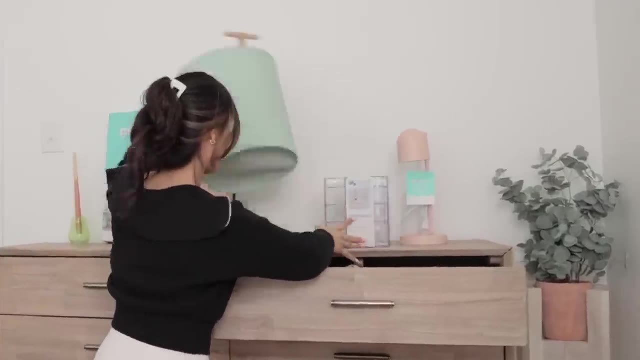 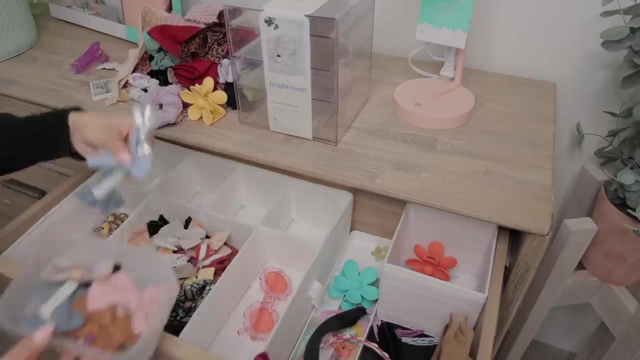 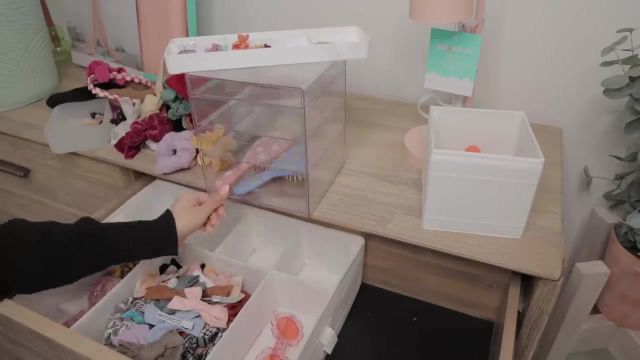 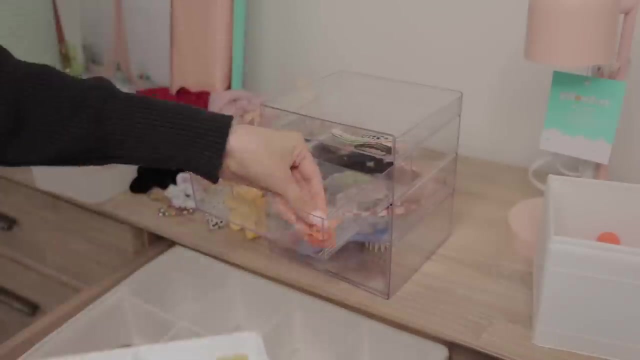 drawer full of scrunchies and I'm hoping it'll look cute just like on here, because, like I feel like it would just be so much easier if I keep it up here, so that way I can just easily get her ready. but yeah, so it is. I don't know what I'm going to do with the rest of it-. 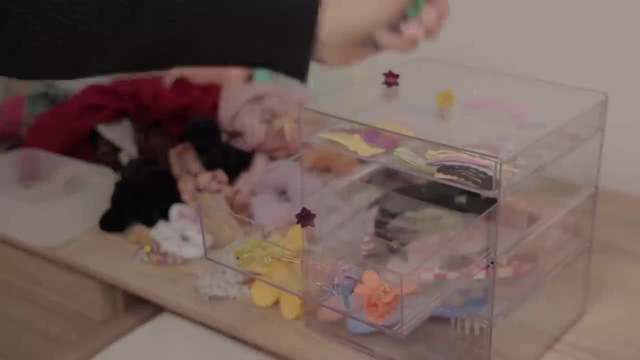 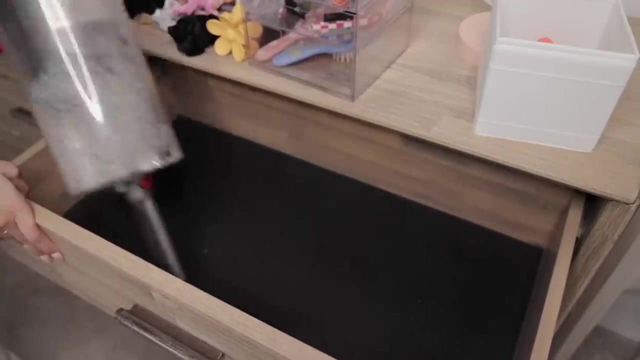 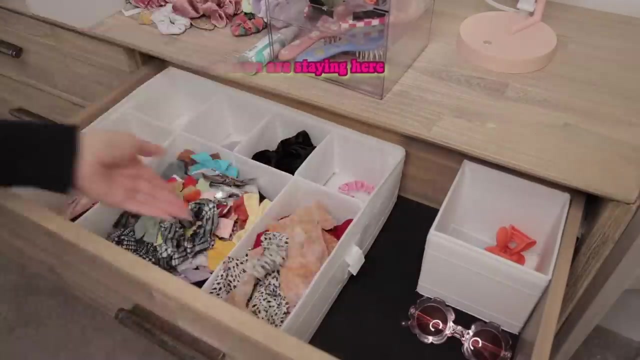 that's the size of this drawer- so that's really perfect. so the drawer is designed to be really big and I like that. it's easy to pull it out and I can just put it in the drawer like this, and this is how you place it. just make sure that the drawer is nice and tight and those little items on the top are just the right size to lay on the desk. 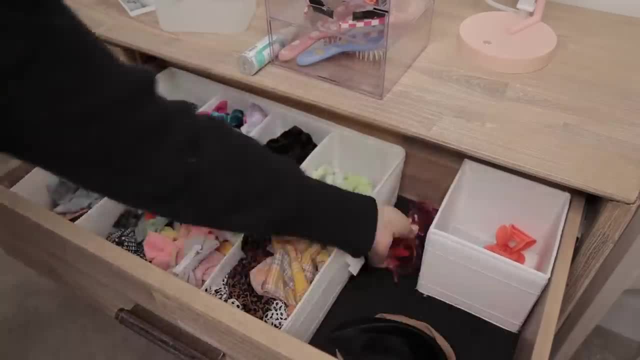 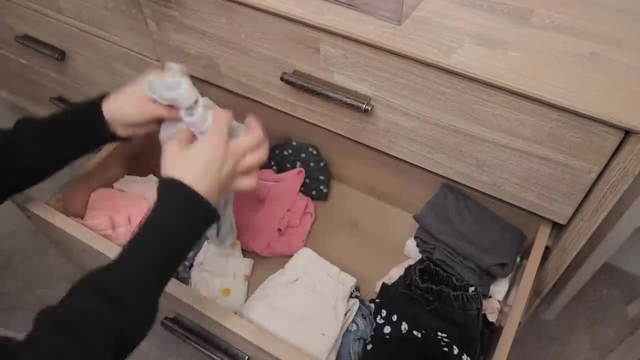 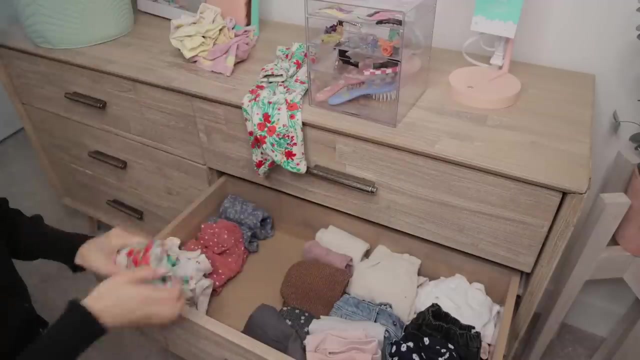 oh. so here's a couple more things to help me create now. here's a few things to make sure that the drawerが, I feel like a number one under the fading sun And our hearts beat faster. now We follow the tracks till we're lost. 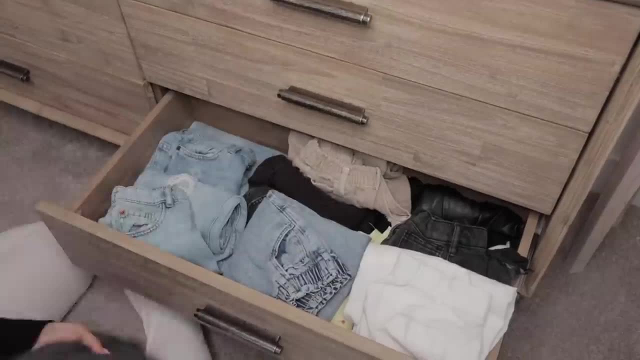 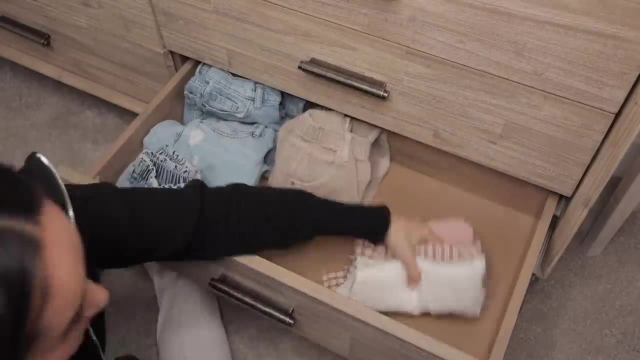 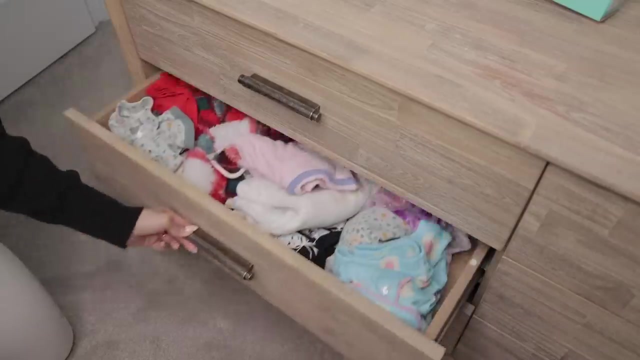 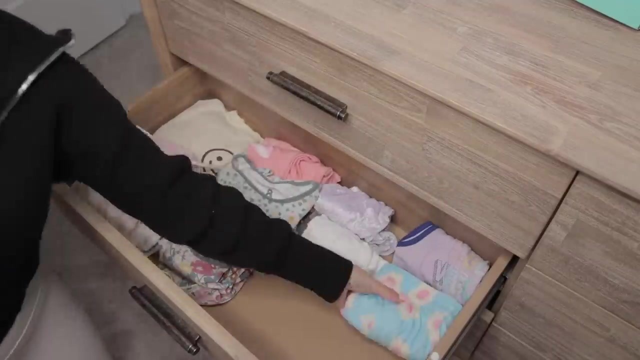 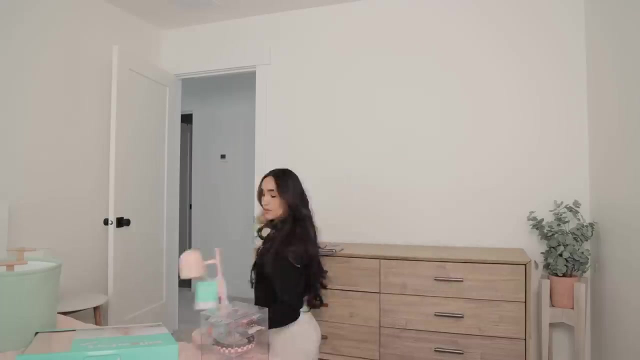 keeping us safe in the dark A long way. down to the same old song: Oh my love, what's on your mind Round and round? open your eyes. Now the dreams are scared. now the dreams are scared, And there's no way back when we run. 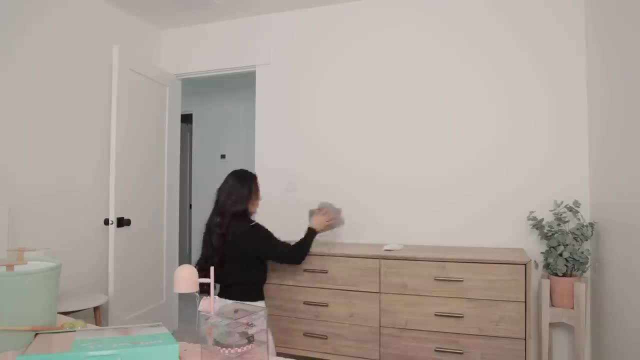 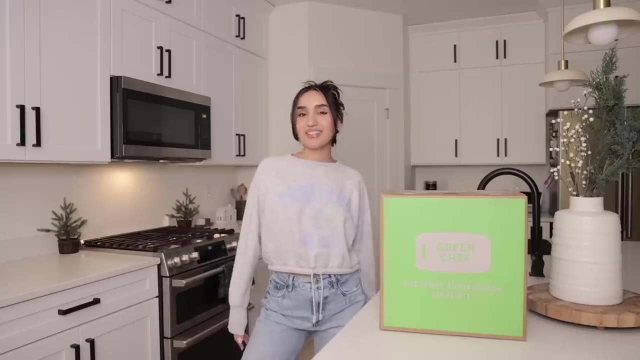 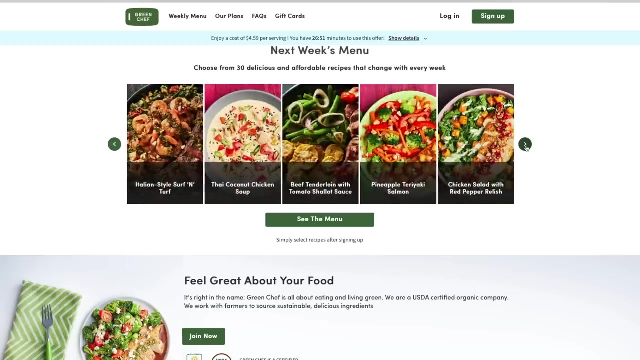 We just gotta break the line. So popping in here to thank Green Chef for sponsoring today's video. So Green Chef is the number one best meal kit for eating. well, With Green Chef you get organic produce and premium protein so you can feel good about what you're eating and how it got to your table. 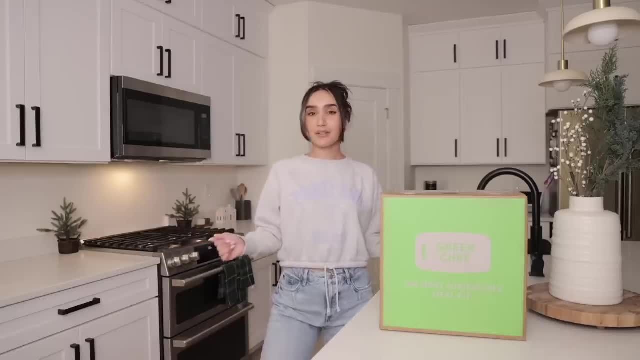 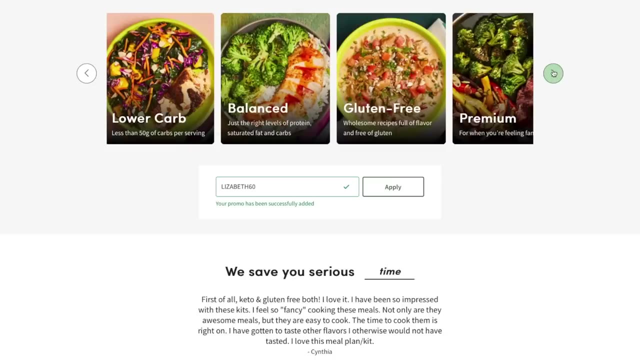 And Green Chef is a CCUF certified brand and they have options for every lifestyle. So they have options for Keto, Paleo, Vegan, Vegetarian, Fast and Fit, Mediterranean and Gluten Free. And what I love most about Green Chef is that I can spend time on other goals. 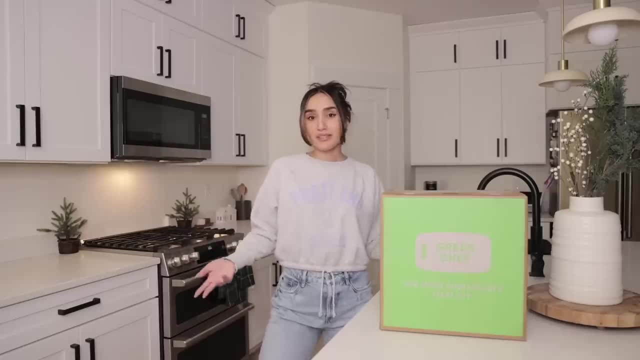 that I'm trying to reach this year and not have to worry about dinner Like today. I've been busy cleaning out the kids' rooms, organizing it. It literally took forever And now I can have a delicious home-cooked meal that I didn't have to plan or go grocery shopping for. 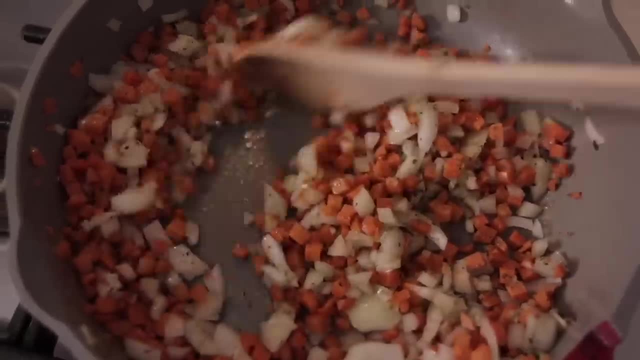 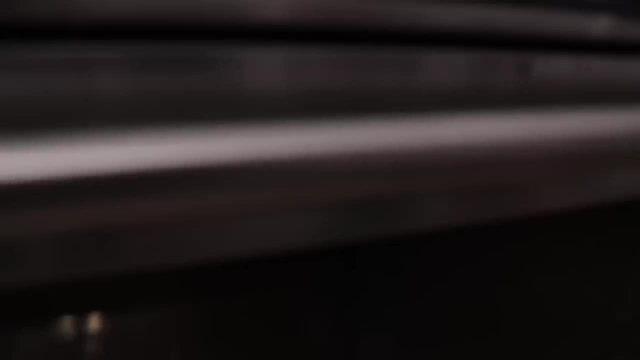 So tonight I'm going to go grocery shopping. So tonight I'm making this shepherd's pie. I love the fact that I can sample different recipes out that I wouldn't normally try out, Like this one, for instance. I probably would never look this one up, to be honest. 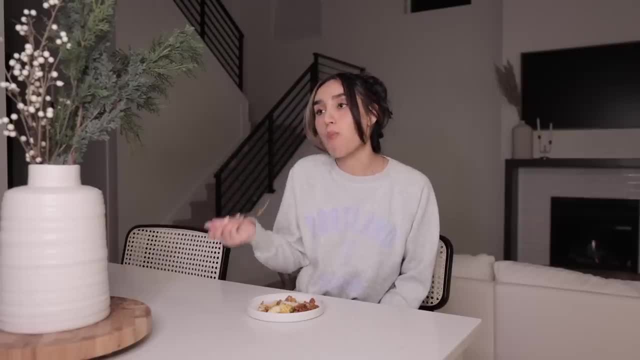 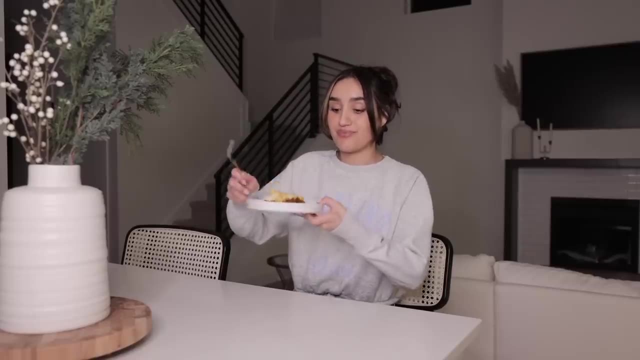 But let me tell you this has become my new favorite build out. It's so warm and homey. This literally looks like I would go to a restaurant and order this. Look at that crust. Mmm, That is like, so warm. 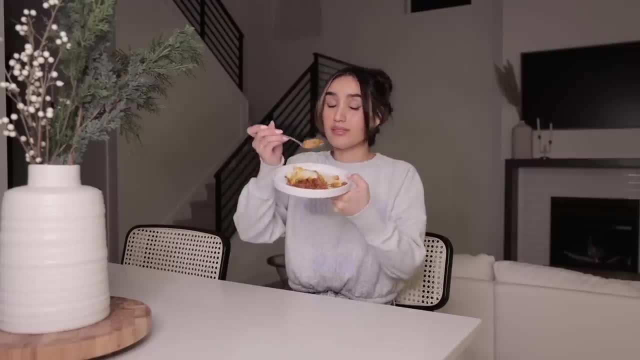 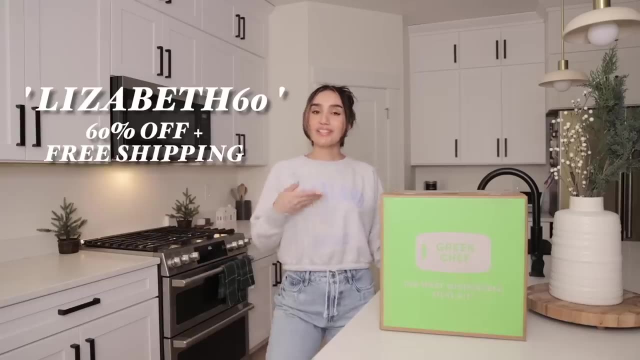 Perfect, It's freezing outside. If you guys would like to try Green Chef out for yourself and see what the hype is about, use my code ELIZABETH60 to get 60% off your first order, with free shipping. Go to greenchefcom for more details. 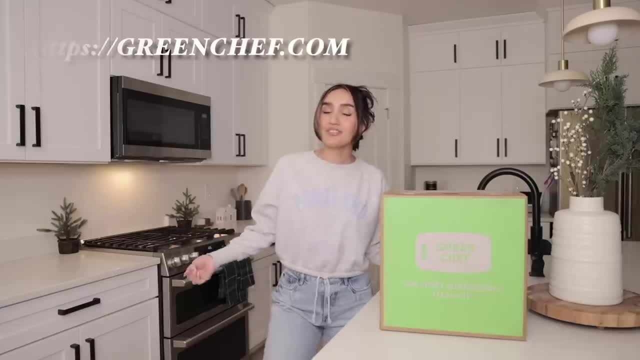 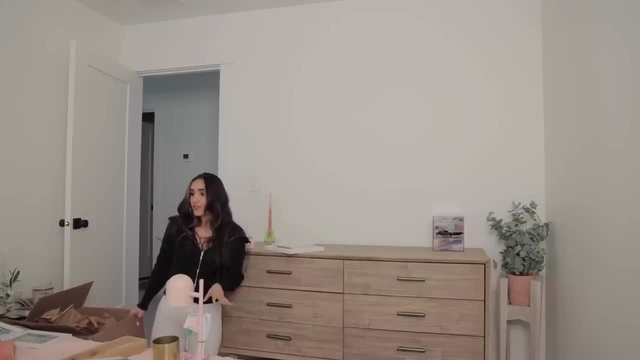 Thank you so much to Green Chef for sponsoring this video. So I just unpacked Emma's bowl decorations from her house. I'm so excited I got my bowl decorations from her last room. Just goes to show, I literally just skipped decorating the kids' rooms. 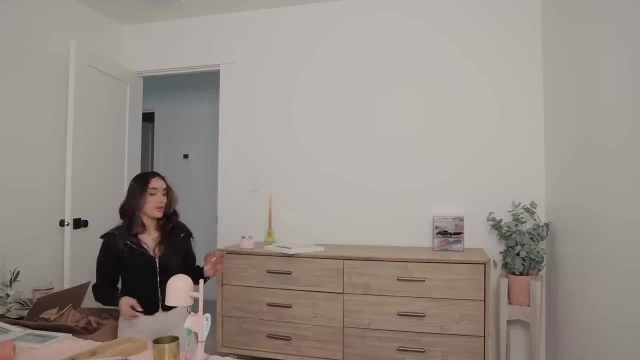 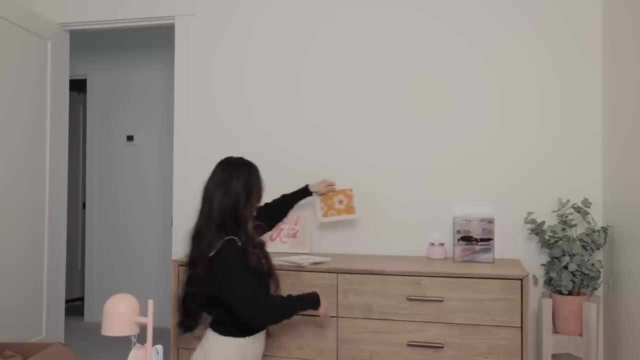 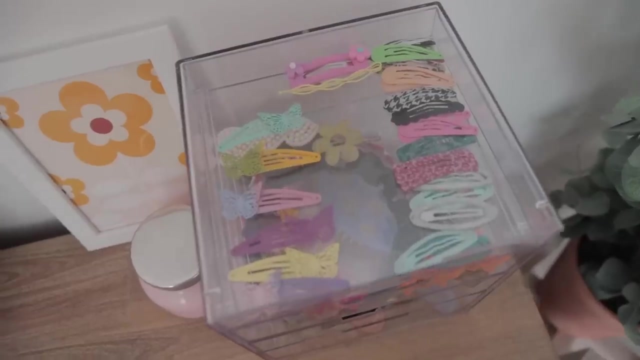 Yeah, I'm going to go ahead and use what she already has. So I'm thinking like a couple of bases. This, I think, will look really cute right here. Cute, No, just not so boring. you know, She has some personality in here. 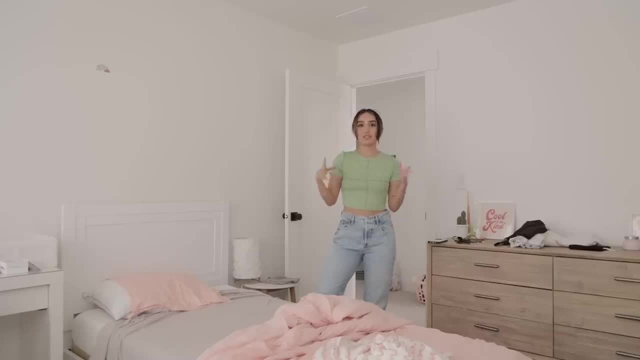 So this side is finished, Day two of this. you guys, I had to stop Because it was already getting dark And then the kids are at school tomorrow, So luckily they're at school right now. So I'm going to go ahead and finish up with Emma's bed. 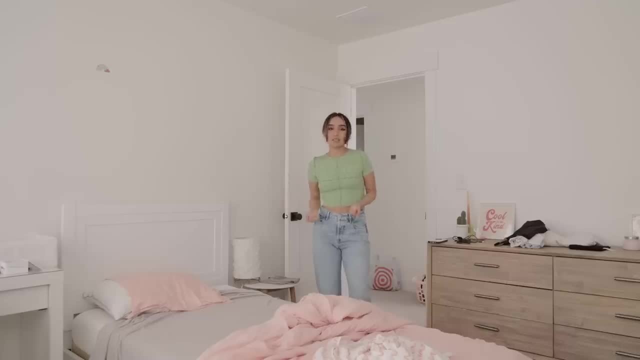 So funny thing with this is that I got her the exact same bedspread. I feel like I do this so often, But something always happens, Like literally like something's always happening to her bedspread where it gets stained And, yeah, I can't use it anymore. 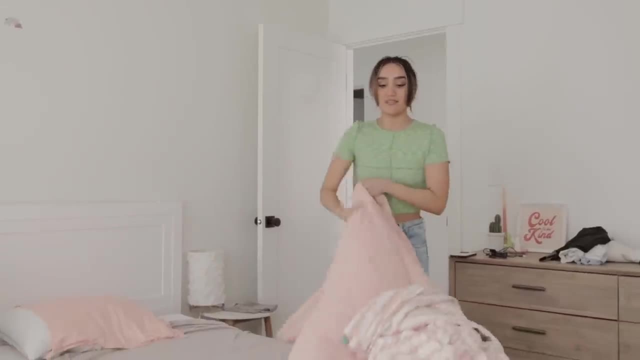 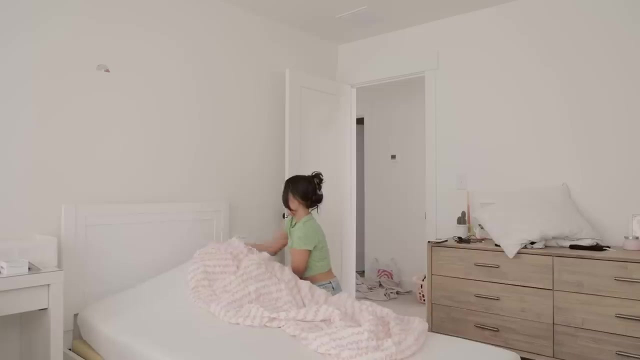 With this big Sharpie stain. But now it's time to like say goodbye, Because there's no fix for that. This is the exact same bedspread that I bought her, Just one that isn't stained. so Okay, I'm just not going to wash her comforter. 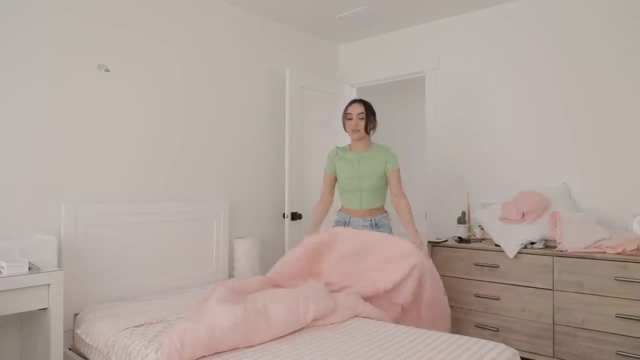 Because she's not going to even sleep on it, Because it's sheet, And I, lowkey, wish I did that with the boys, Because theirs is all like wrinkly now, So I'm like dang it. Oh, it's so brand new and perfect. 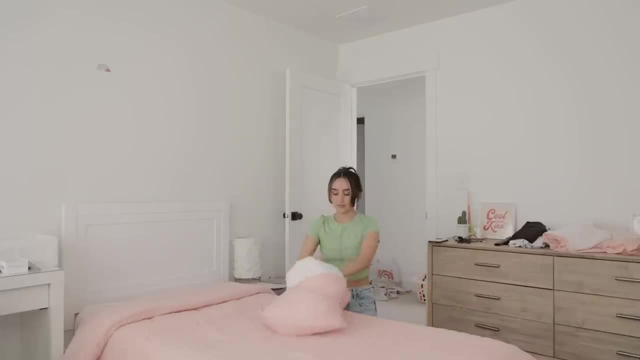 And then I just have to look for her rainbow pillowcase And then we're going to move this bed, Because one thing about Emma is that she's a hamster, Like literally anything that's kind of like she sees as value in this house. 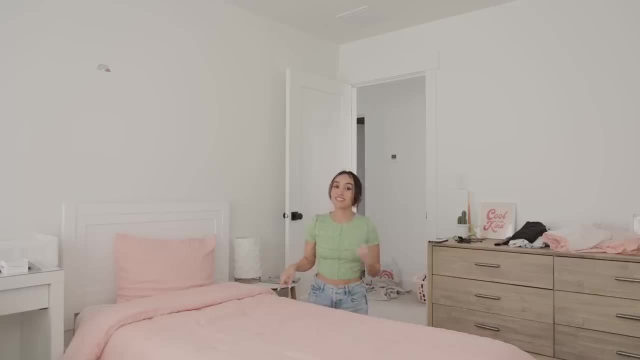 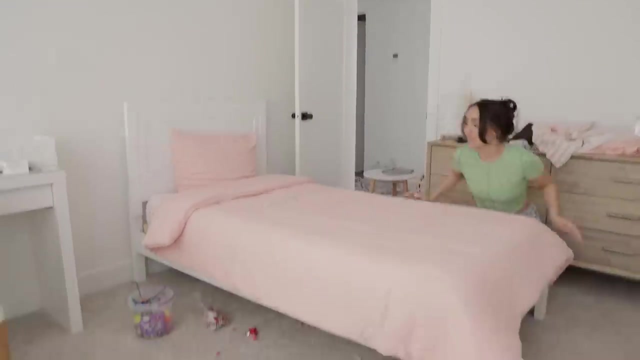 She'll like hide it under the bed. She'll put it under her desk in the closet. So we're going to find some interesting stuff here in a bit. Oh, it's actually not that bad. You know what I actually think. the last time I was in her room I cleaned it. 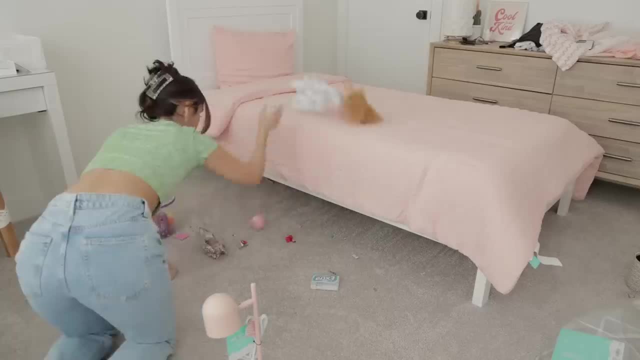 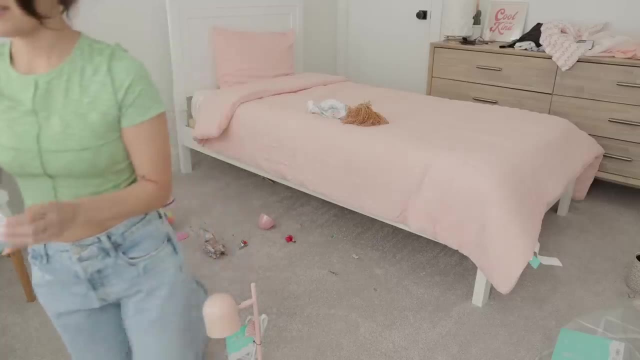 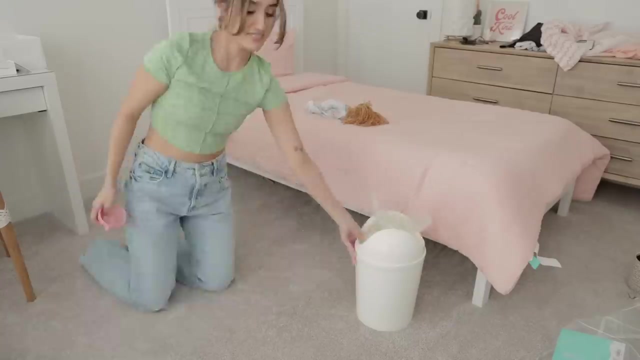 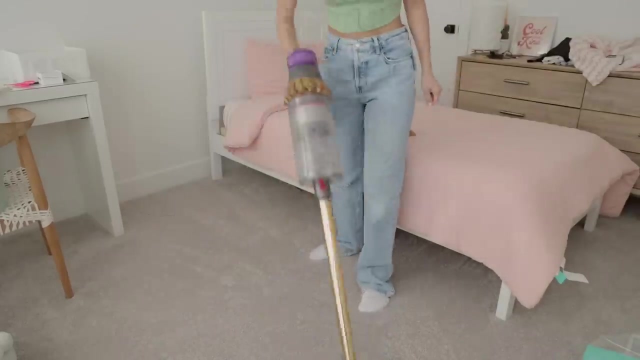 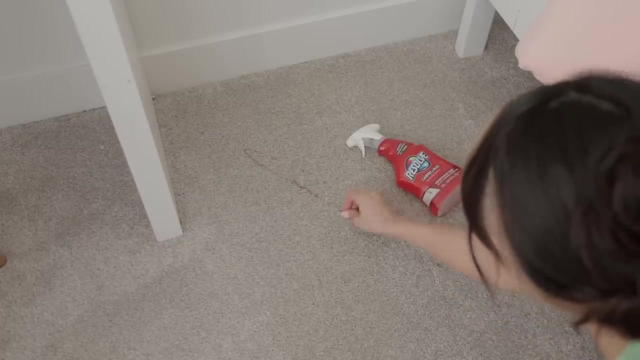 But look, Look at that spot, This is my gum. I always keep in the car And she always takes my gum, Brad. And then, of course, this girl has glitter glue all over the carpet, So I don't think I could peel it off. 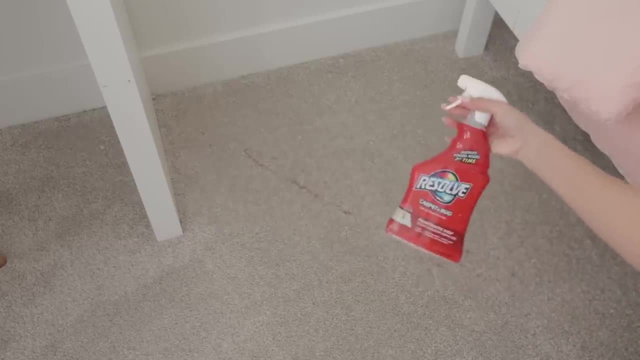 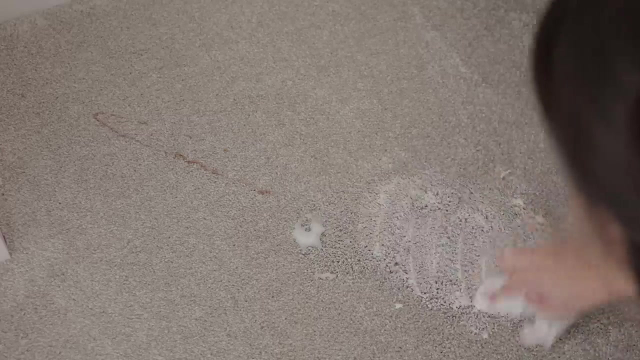 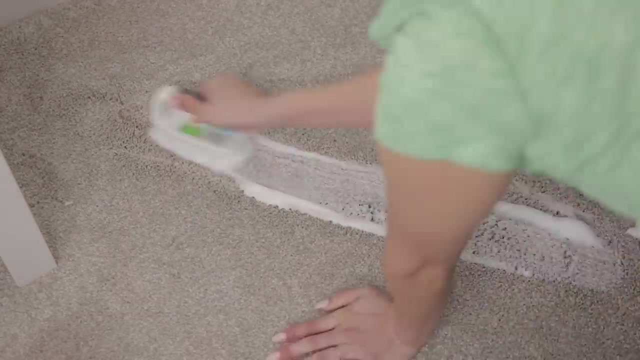 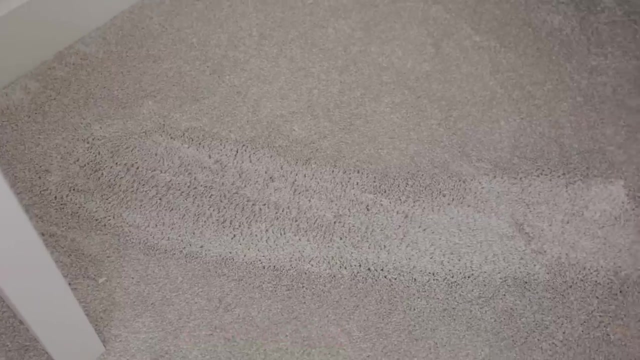 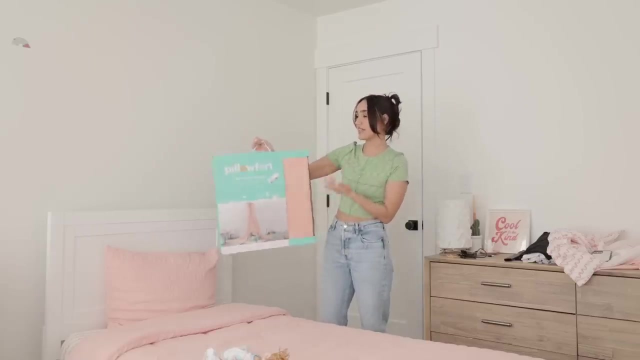 So I'm just going to try to scrub it off with the carpet cleaner. So next up I got her this cute little canopy. I know it's pink, So I'm going to kind of see if it's like too much of the same color as this. 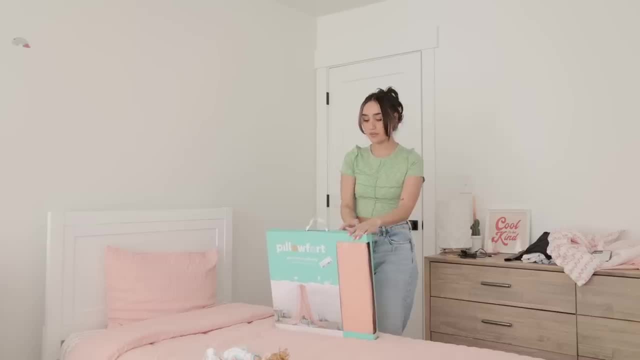 Because if it is, I think I'm going to have to move this somewhere else. Okay, So this is definitely not going to work on her bed, But I think we should try to make it work somewhere else. I'm thinking. I think I'm just going to keep it above her bed. 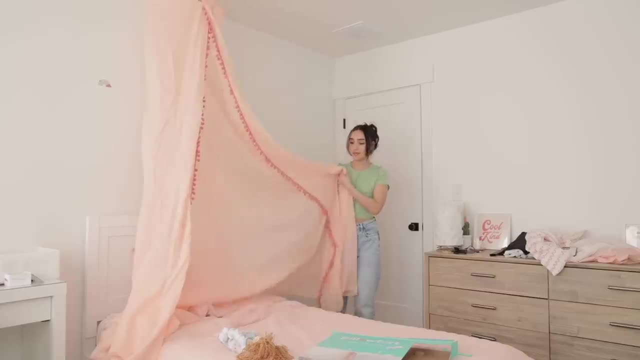 Because I feel like it'll look best here, But then change over. I'm going to have to play comforter. Okay, So it's up, Looks really pretty. Of course I have to steam it, So that'll get done. Tuck this behind the bed. 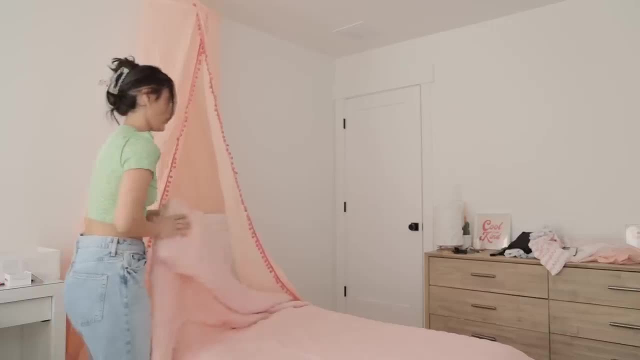 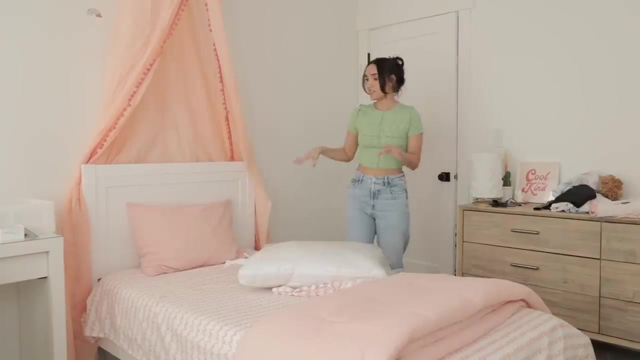 So cute And then, for the time being, We're going to fold this down And do you guys see the vibe? I think it's really cute. I think what will look really cute is if I put a quilt on top And then like, obviously not pink. 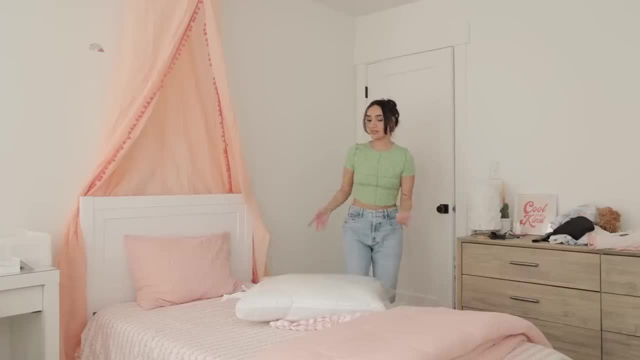 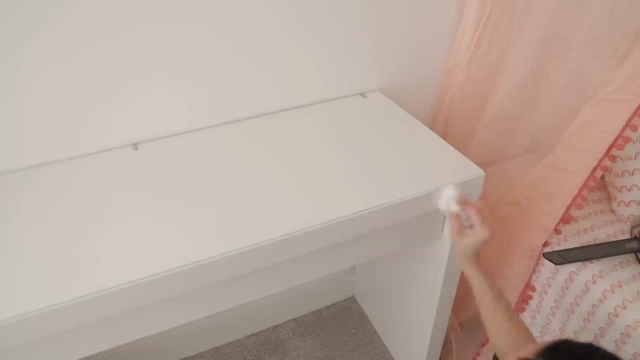 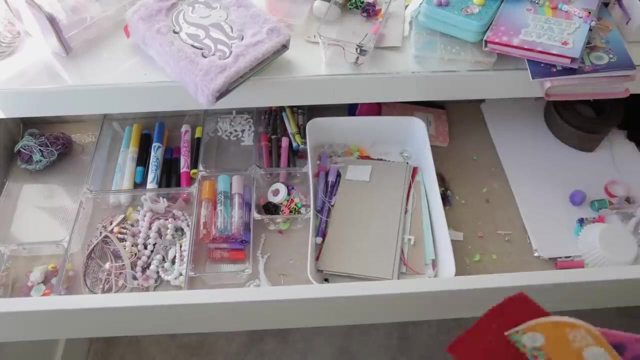 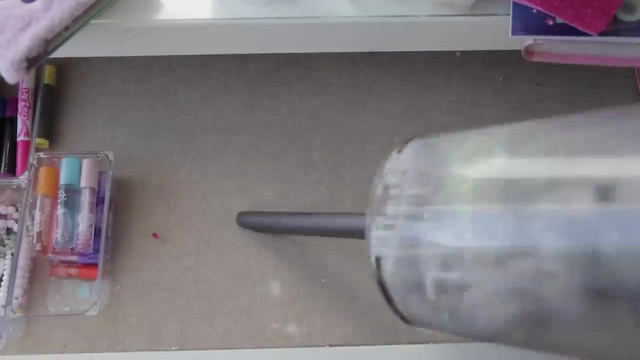 Because there's too much pink going on. Okay, Perfect, Okay. Oh, my goodness, I can't believe this is going to work If we fold down the sides. It's going to be like this. It's going to be like this. 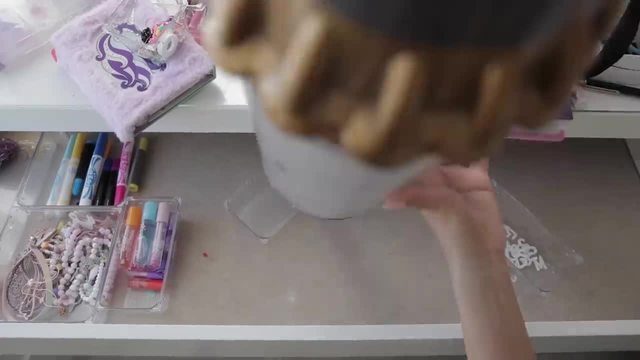 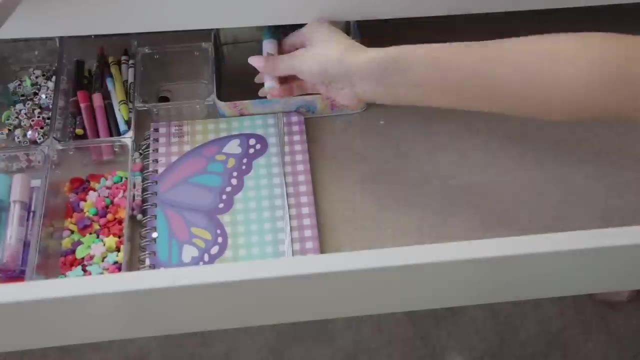 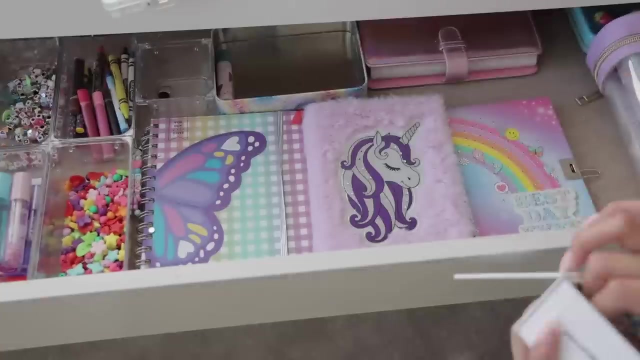 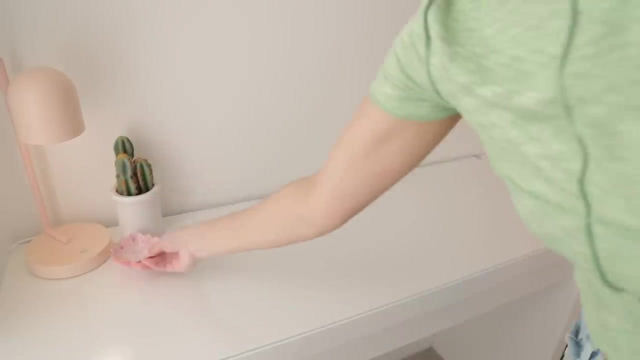 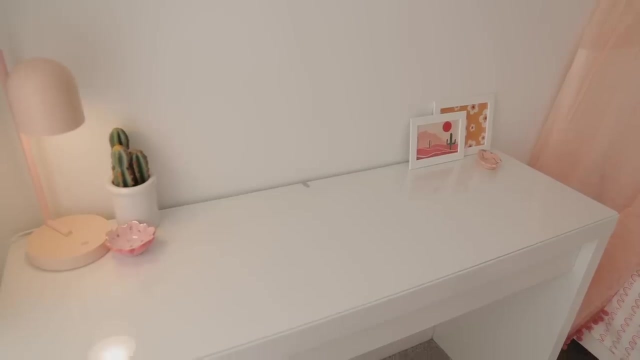 We're going to have to bend the sides a little bit. Okay, it literally looks so good like i basically only bought that lamp. i had everything else and i feel like it's looking so good. let me show you what the inside looks like. i got all these. 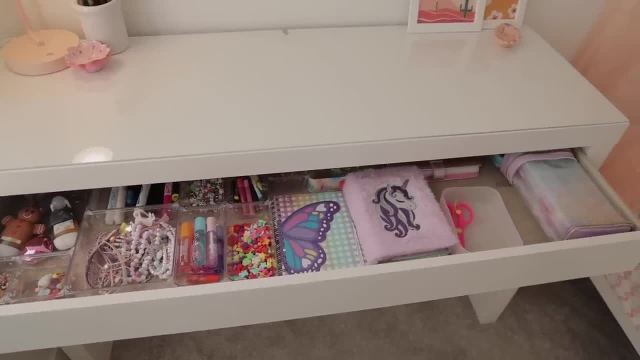 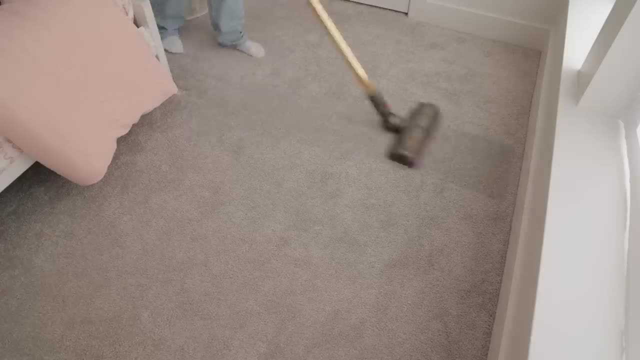 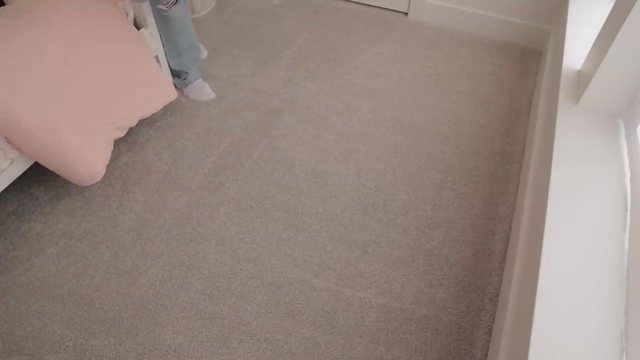 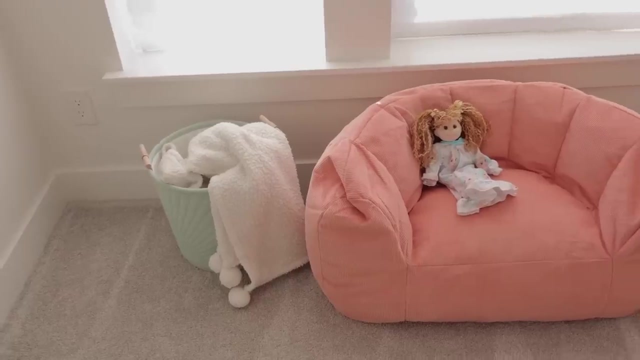 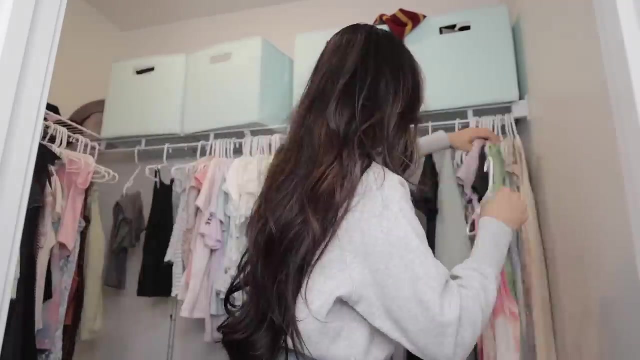 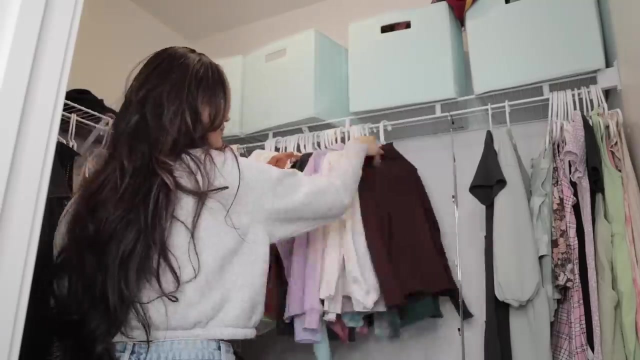 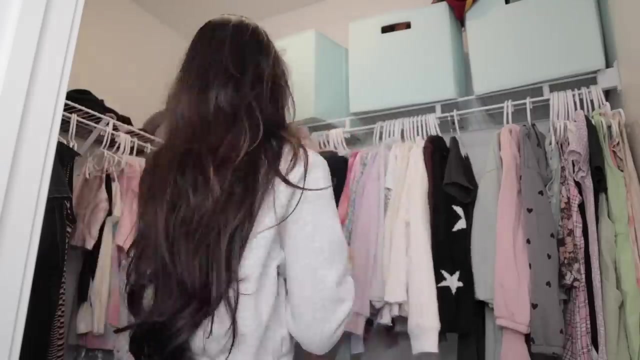 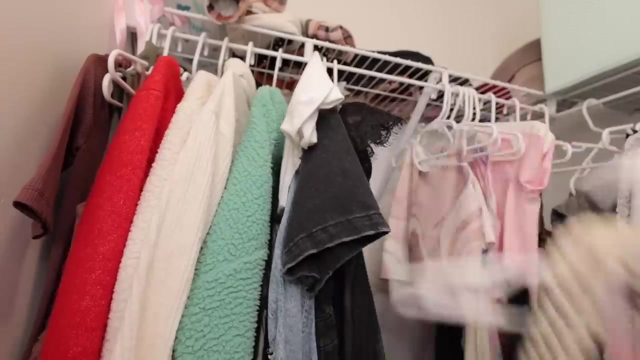 like acrylic clear things from amazon and some are from target too, floating rivers upstream. the things that you said, tell me and be honest. tell me, did you know that you would believe in me, just like the winter snow? tell me and be honest, tell me. should i know that you'd be leaving me? so 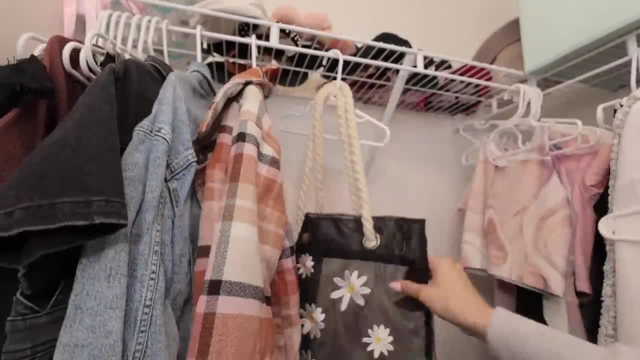 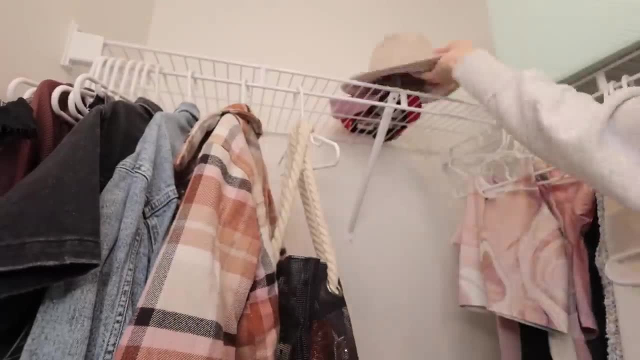 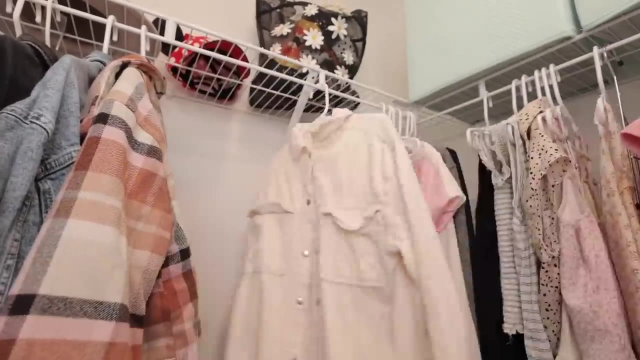 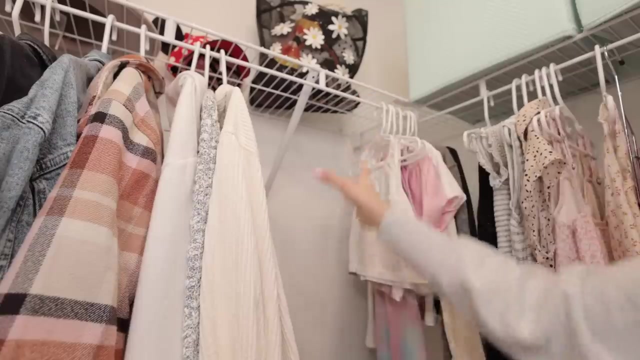 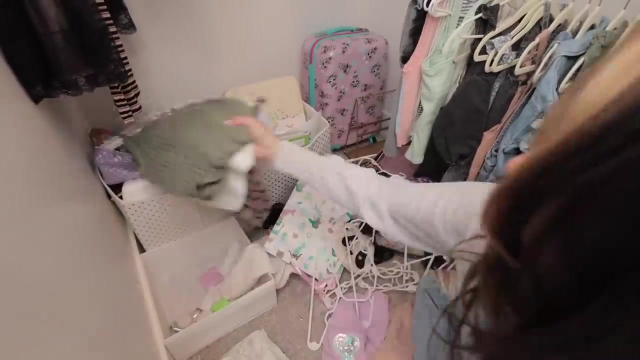 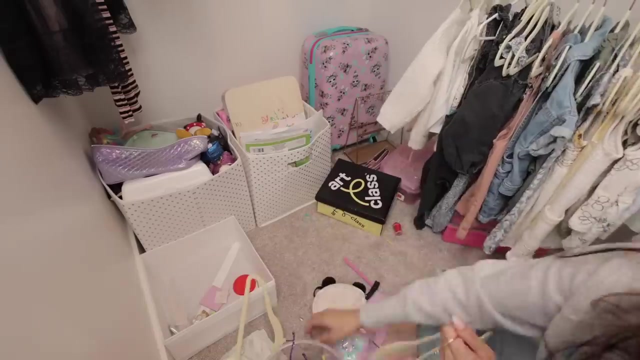 pained, i think, this big empty space. i want to get like one of those little closet things you can put right here and you have like more drawer space. i'm definitely gonna do that here. this is like the haven of my house. i don't know what i'm gonna do with all these things. 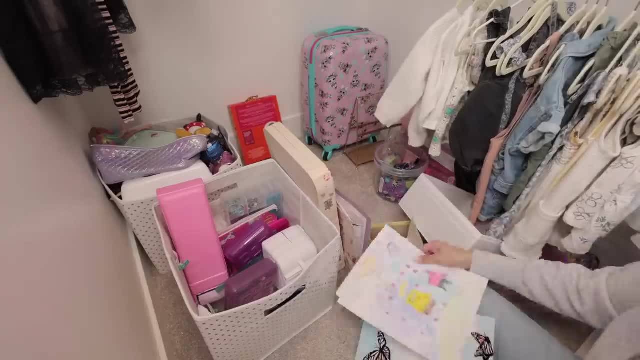 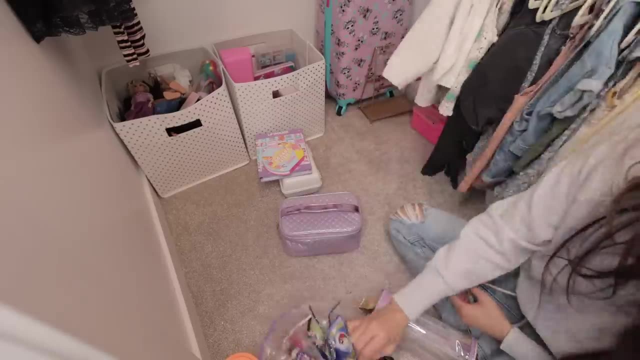 i've been thinking about this for a few years now. i thought i'd be trying to make a house. i wanted to make a house like a house, but the thing is that i've got a lot of work to do, so i think i'm gonna do a real house. 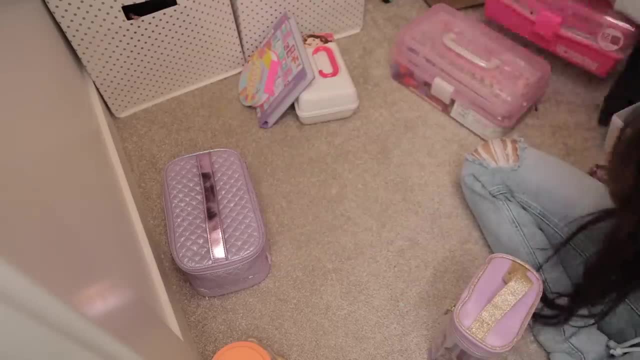 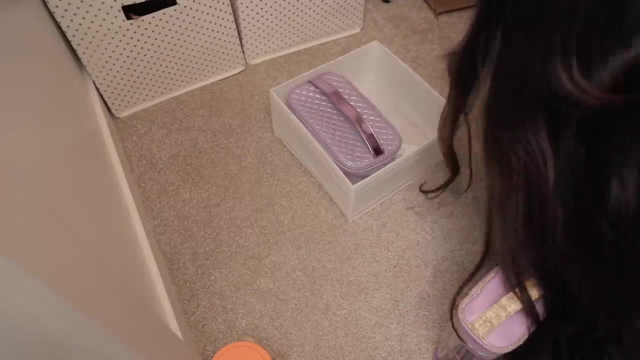 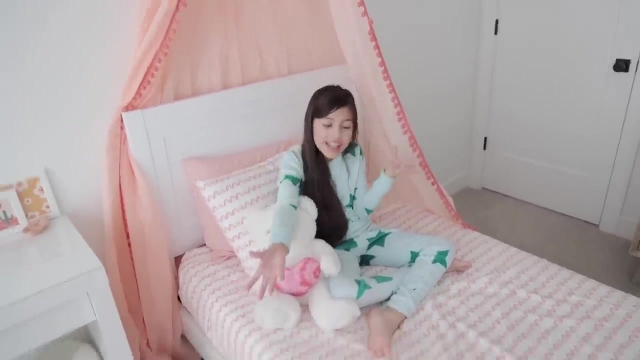 i'm not sure if my house is gonna fit in there, but oh well, it's gonna be nice That you believe in me. So painfully quiet and slow. What are your thoughts? My favorite thoughts: I love the thing bag And I love this little thing. I don't know what it's called. 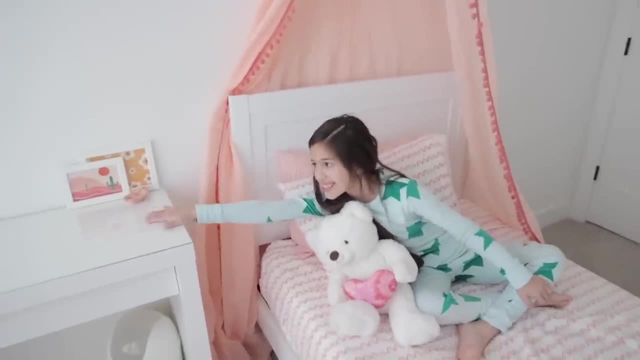 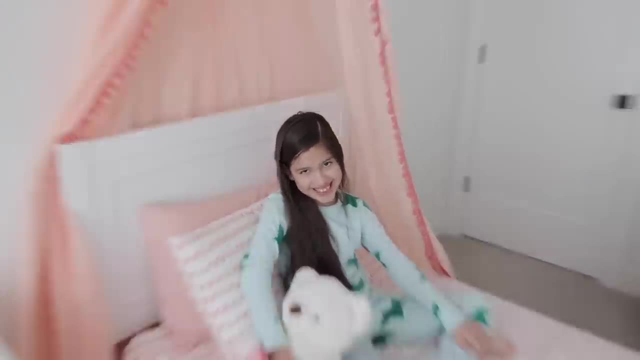 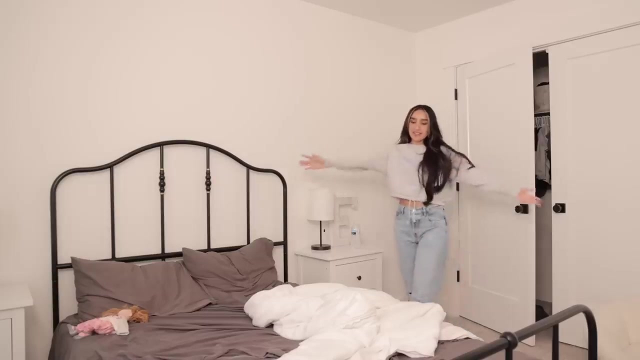 And I love the clean of this. Oh yeah, because it was so messy And you know what we found? The glitter thing. Alright, guys, so now for the boys room. So, as you guys can see, I got the new sheets, new pillows And a bed, because they've had the same bed. 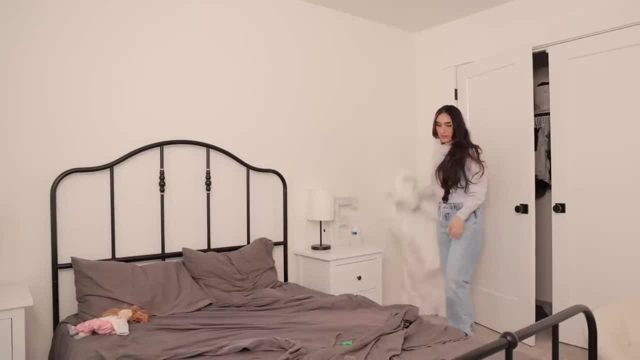 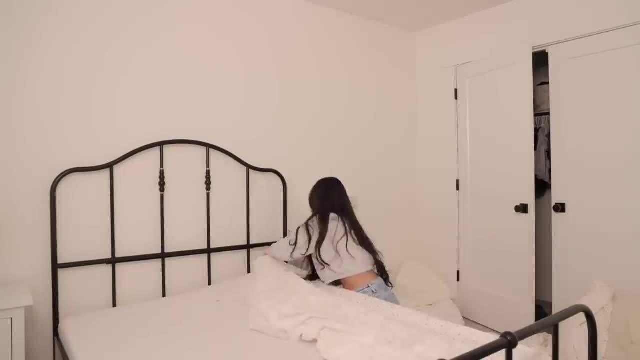 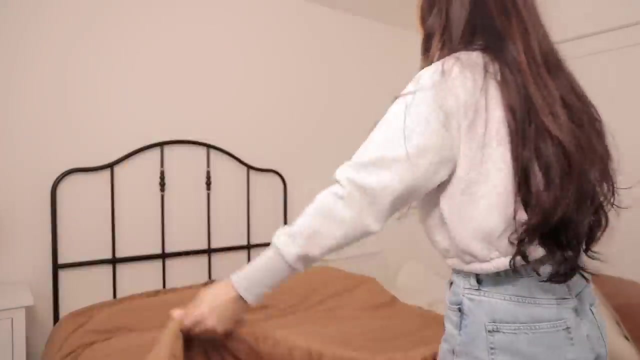 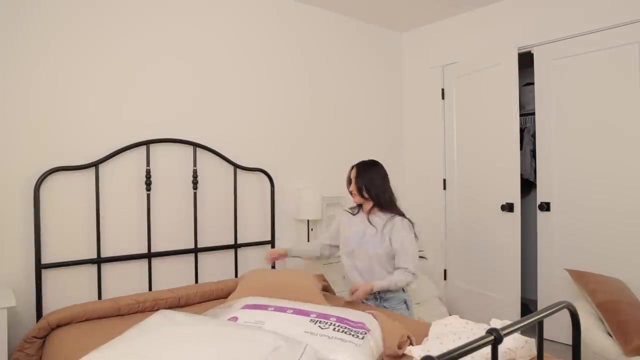 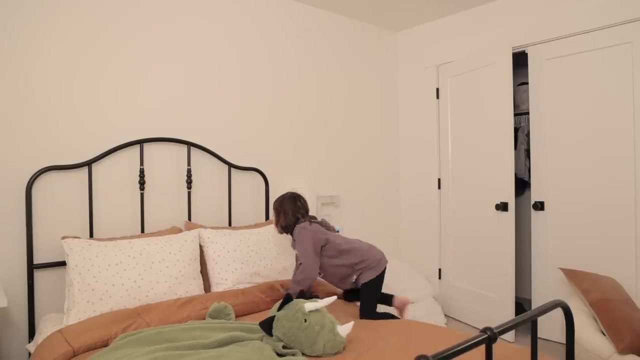 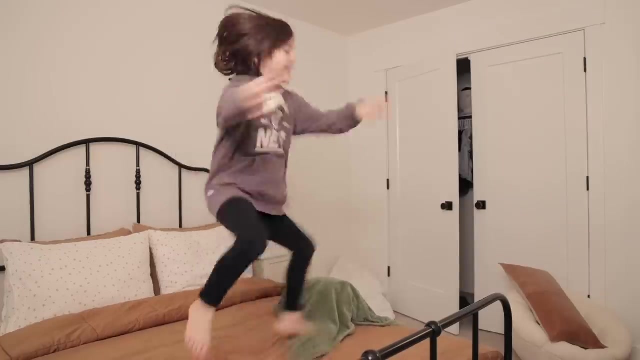 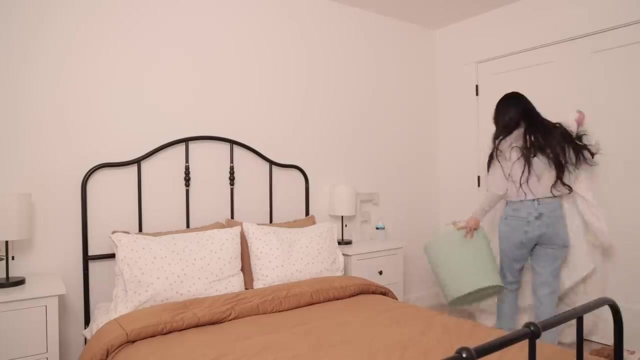 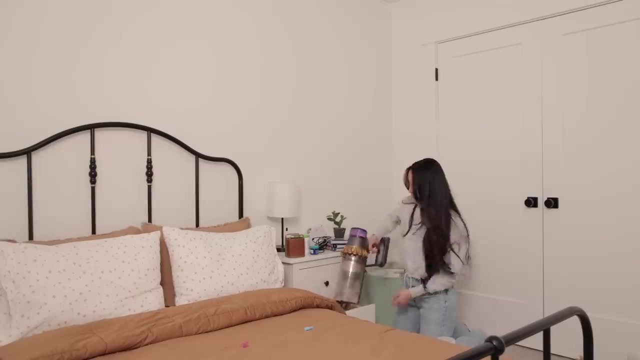 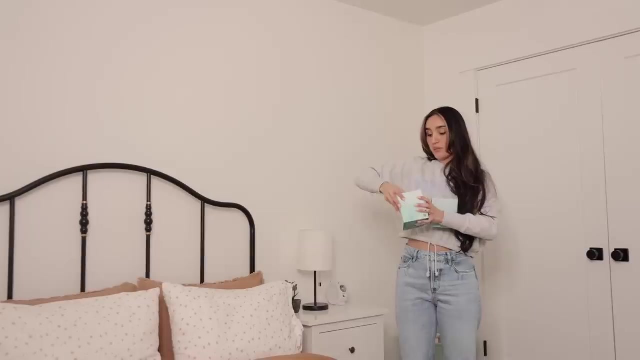 Bedding forever. So I'm going to go ahead and take off everything. What do you think, Zizi? Good, I guess you start. Is it bouncy enough? still, No, You guys have kids that pick their boogers And put it on for insurance. 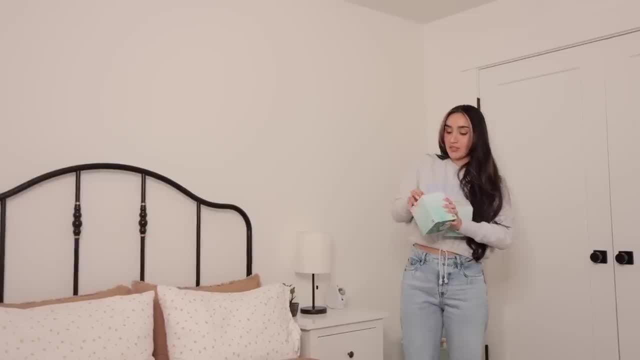 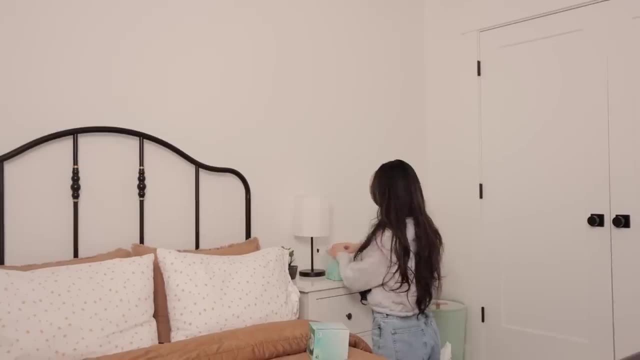 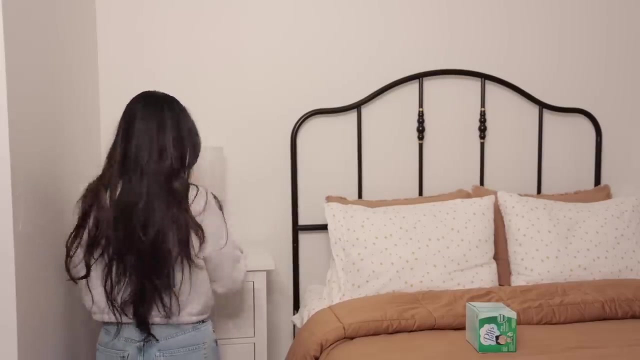 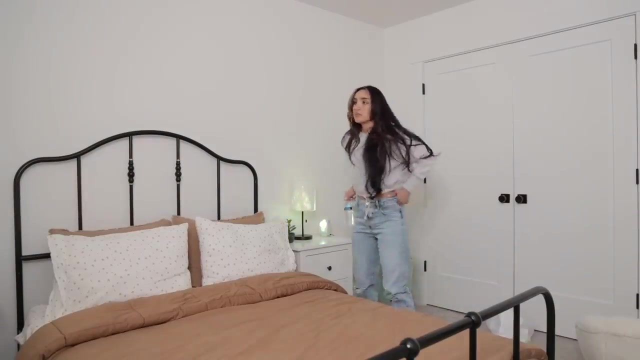 Walls and all that stuff. Definitely get some tissues. I hope, I really hope this works. I don't know if it's a hat, But I'm assuming it will be Okay. It's pretty much done, Guys, I definitely need to get the boys Some more decor in here. 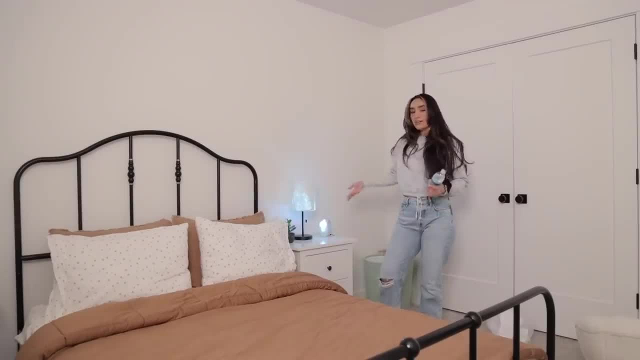 But all in all, They got a new bedding. They got a new bedding And they cleaned their nightstand too, And there's no boogers on the nightstand, So yay. So all I have left to do now For their room Is vacuum. We know the boys need some of this.